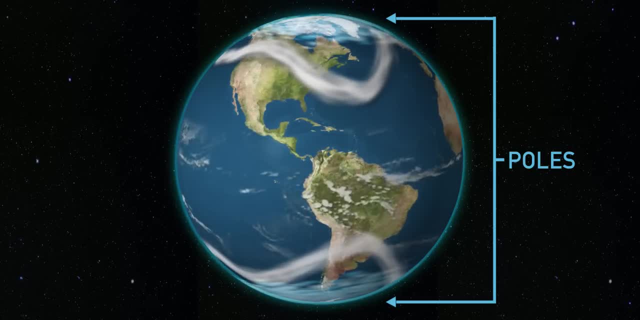 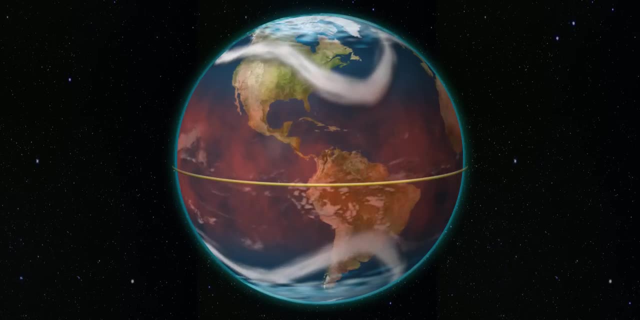 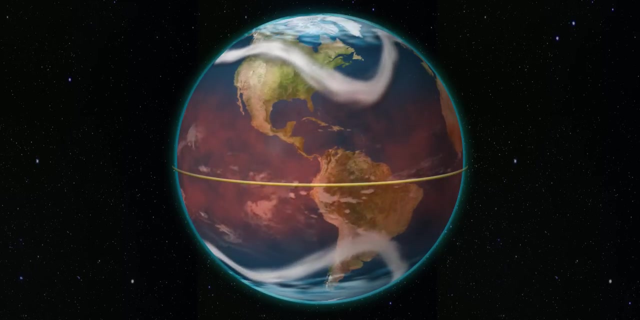 east to west, around the top and bottom of the planet. So we've got cold air on the poles and warm air at the equator, and the jet stream is basically where those two air masses meet. Now, if there was never any exchange of air between these masses, the poles would get colder and 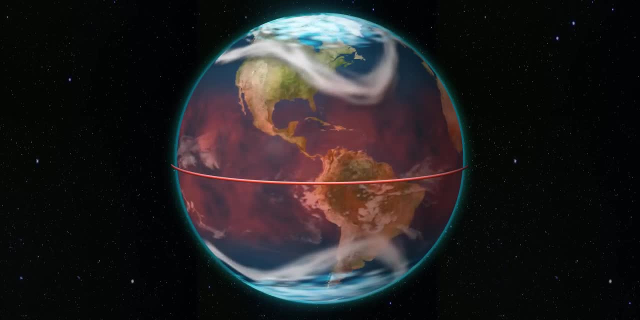 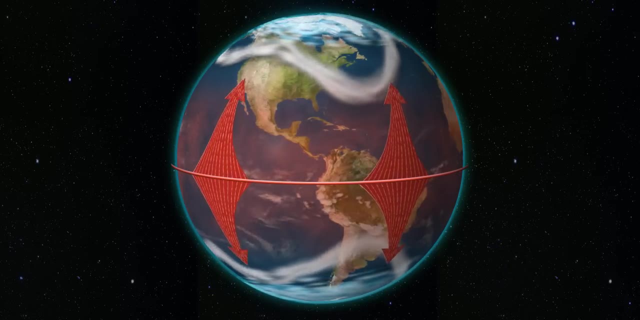 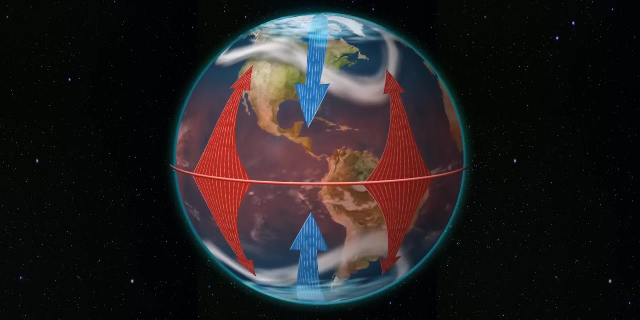 colder and the equator would get hotter and hotter. but temperature is the same. So we have always trying to find equilibrium. So warm, moist air masses move out from the equator towards the poles and cold air pours from the poles towards the equator, The moisture from the 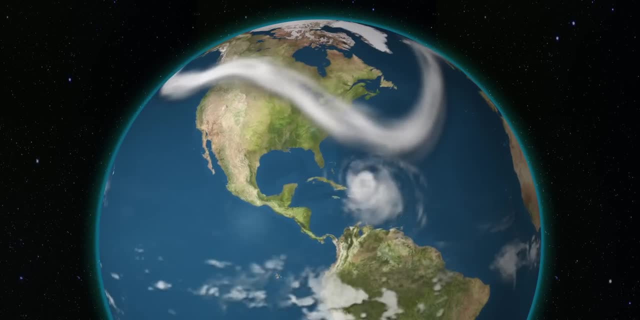 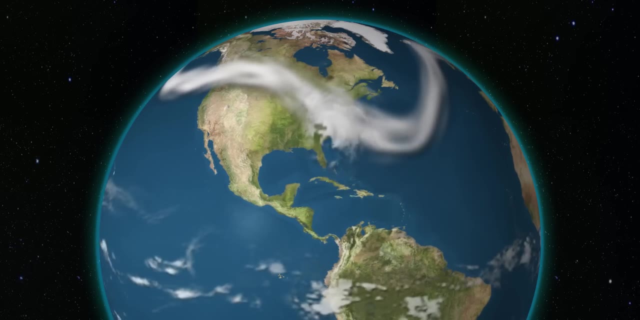 equator moves out sometimes as a hurricane, typhoon or tropical storm, and then gets entrained in the jet stream and starts moving from west to east And the arctic air travels down over the continents and back to the equator. So we have this band of moisture moving around the equator. 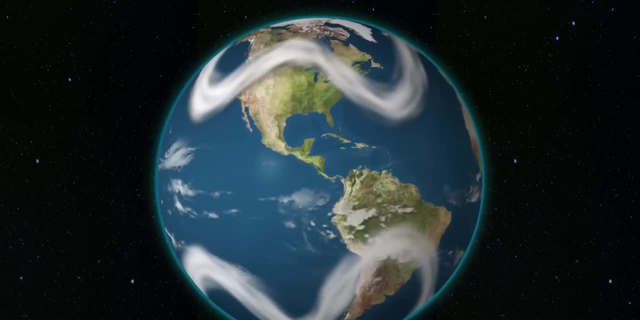 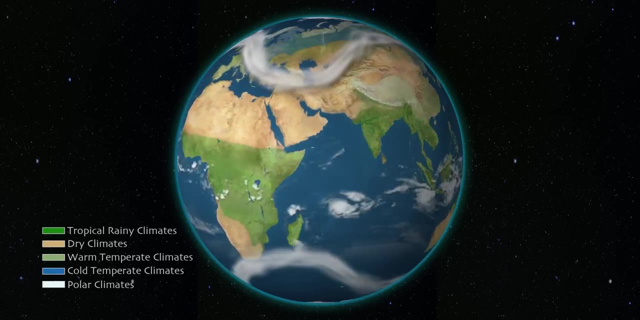 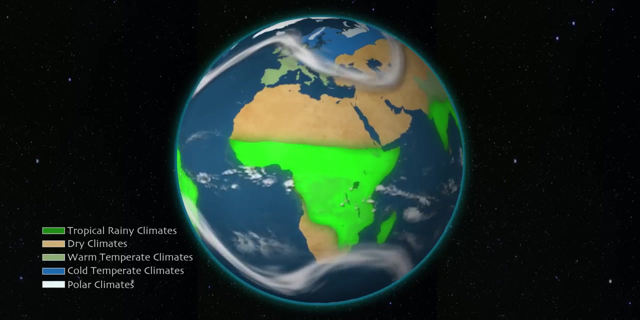 and brings cold weather. The areas by the coasts get less cold air because the mass of the ocean acts as a temperature moderator. So this is how the climate zones are created. We've got wet and seasonally wet tropics in this band around the equator. Then we have the subtropics that are 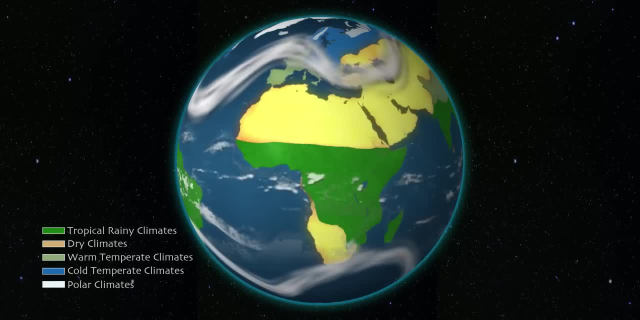 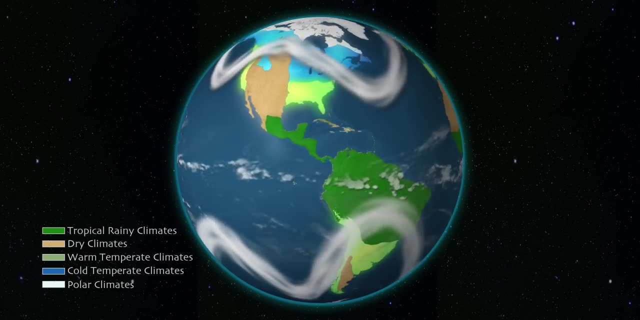 typically dry out from there to what we call the tropics of Cancer and Capricorn at around 23 degrees. Then we hit the temperate zones, which are usually dry out from there to what we call the arctic air masses, which get hit by the jet stream and are cooler and wetter As we move. 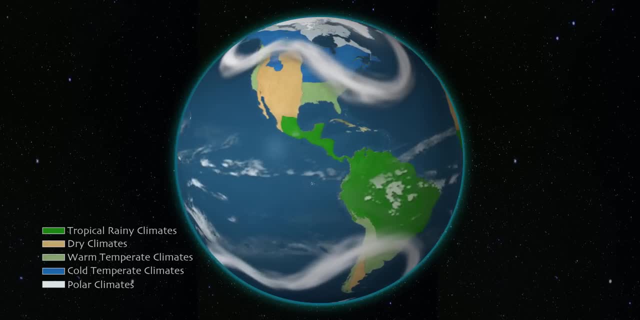 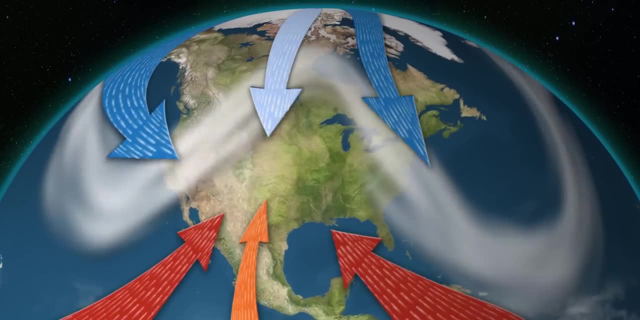 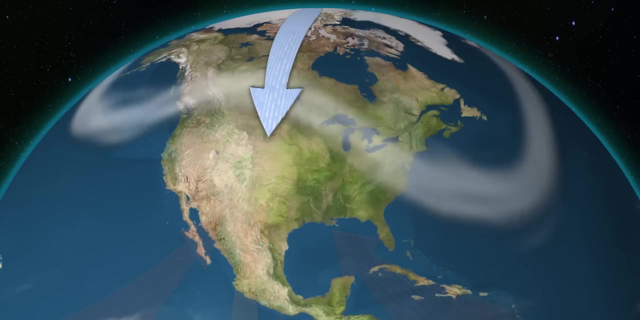 higher. we hit the arctic circle in the north and mostly ocean in the south. We can see that when we zoom into North America there are these different air masses that influence our weather and they basically take turns with each other. Sometimes that arctic air mass comes down deep into the. 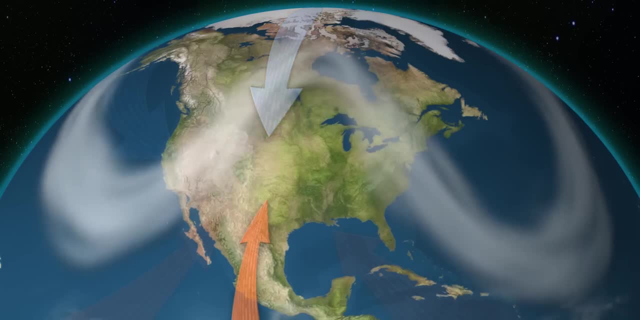 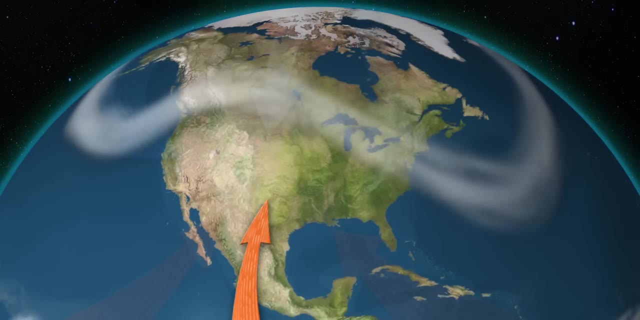 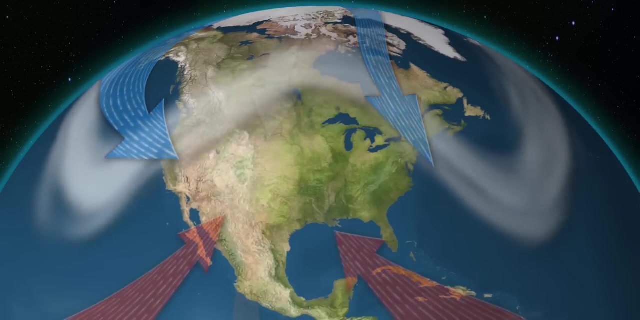 continent and causes a cold snap. Sometimes the hot and dry air builds up in the interior of the continent and builds a dome that the jet stream just stays up above. Sometimes the jet stream brings cool, moist air as rain and snow over the continent, and sometimes tropical air comes up and 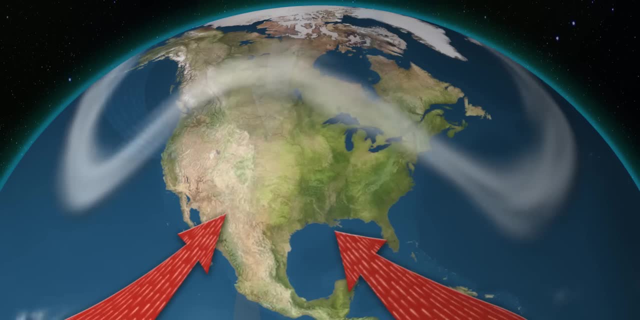 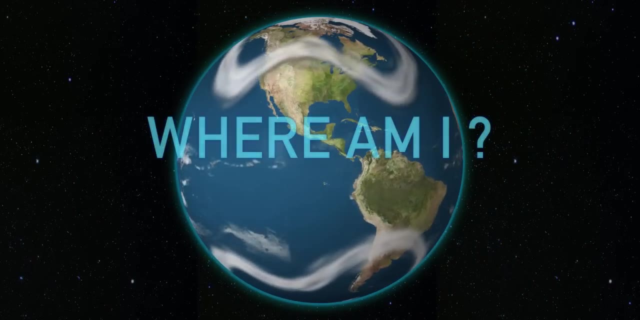 gets entrained in the jet stream, bringing warm rain on the coasts and interior. Now let's go back to our original question: Where am I? You can better answer that now that you have some context of where you are within the global climate. You can better answer that now that you have some context.